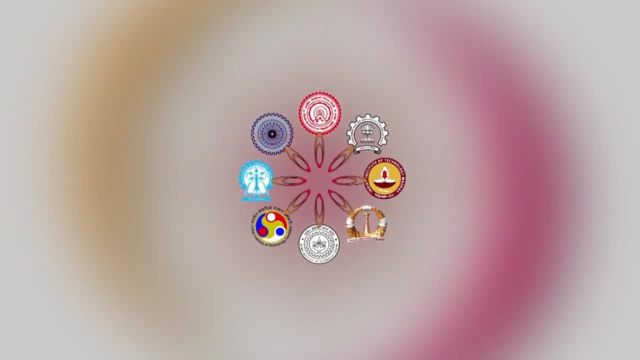 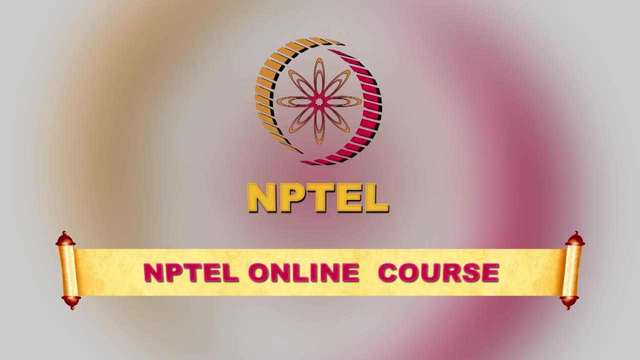 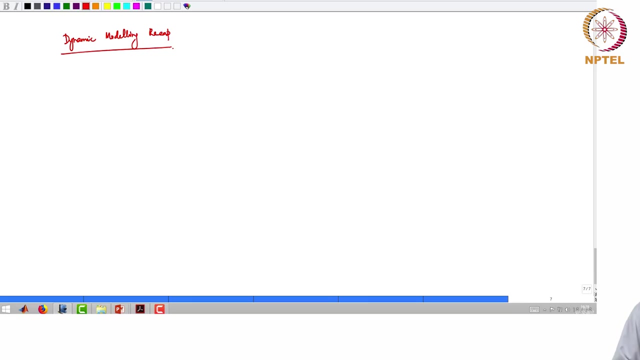 So in today's video I will do a sort of complete recap of all the concepts of dynamic modelling. dynamic modelling recap. So where did we start with dynamic modelling? So some simple basic kinetic models, Michaelis-Menten, we did briefly look at Hill and 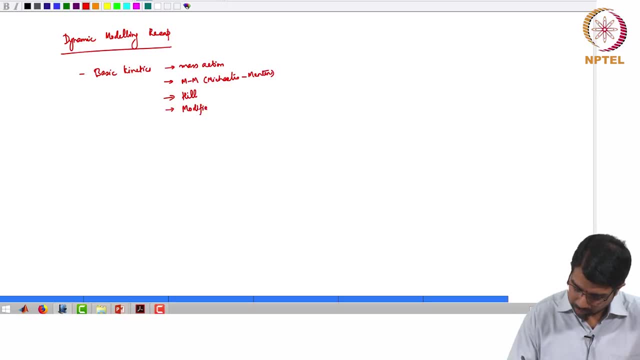 Various types of inhibitions. okay, So essentially the logic was the same in all cases. draw sort of wiring diagram, figure out what are all the interactions, qualify every interaction with some kinetic equations and then assemble a bunch of equations differentiate. 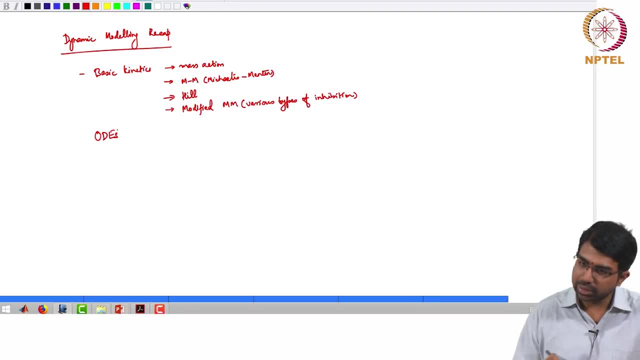 So then ODEs, right. How did our ODS system look like? Right, where x is your m cross 1, vector m equals number of metabolites, S, which is the structure that is of theкрosi Pharm, poussib khaand X. price is apos, point, Osan, okay, So 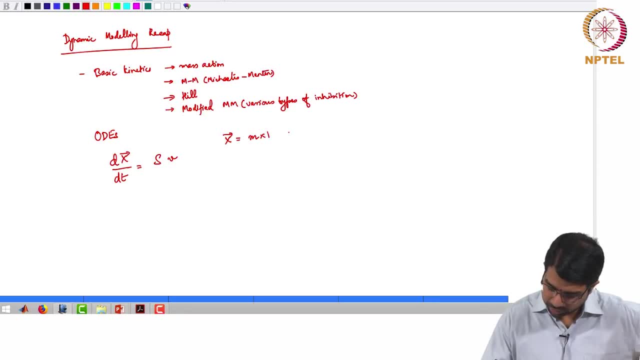 here is your Christian. What is 없? Hold on Just a minute Vy. What is the Egyptian Vy? Hj for Lieu we have K Okay, deal in with the kineticsbrook permutator. Politically, we did. 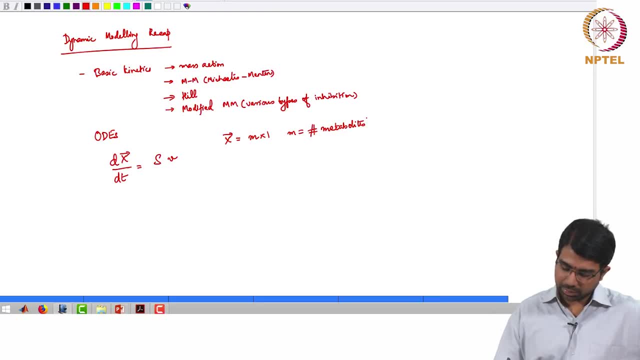 So that was what we decided, like I was going to do after Today. how would your equal to constant physical length S stoichiometric matrix which has negative coefficients for reactants in a reaction and positive stoichiometric coefficients for products in the same reaction? 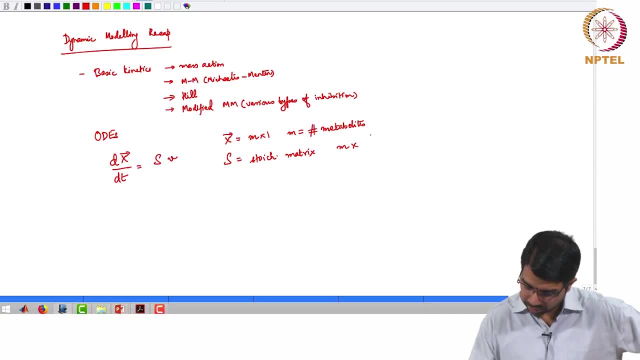 So this is an M cross N or let us say R matrix, where R equals number of reactions and V is obviously going to be an N cross 1 vector or R cross 1 vector. So if you have all the reactions written down for any given system, let us say you have. 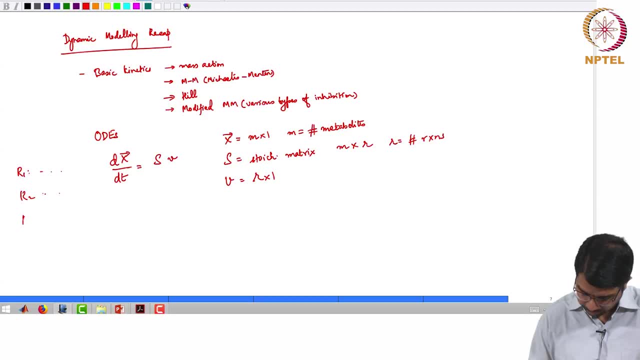 R1, R2, R3 and so on, with involving metabolites. let us say a simple example would be DABCD by 2.. DABCD by DT equals some minus 1 plus 1, 0, 0, 0 minus 1 plus 1, 0, 0, 0 minus 1 plus 1,. 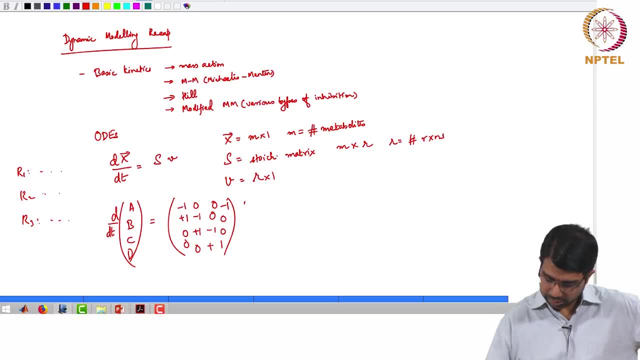 minus 1, 0, 0, 1, right into V1, V2,, V3,, V4, I have same number of metabolites and reactions. So what are my reactions if I were to reconstruct from here: A giving B, B giving C, C giving D and A giving D. is that clear? 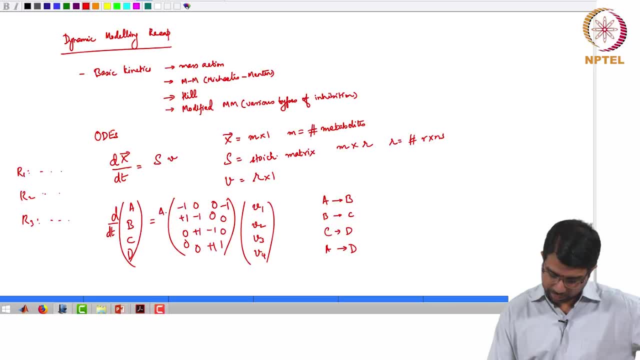 It is from this matrix, right? So this matrix is essentially- you have to think of it- as A, B, C, D and V1, V2, V3, V4, where the V is correspond to everything, Every given reaction. 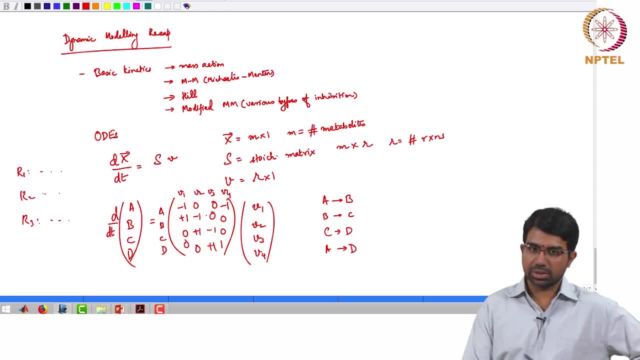 V1 is the rate of R1,, V2 is the rate of R2, and so on. What is V1?? What is that? DA by DT. DA by DT. What is that? DA by DT. DA by DT. DA by DT. 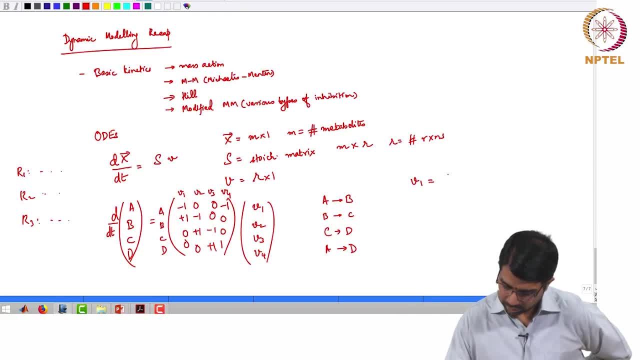 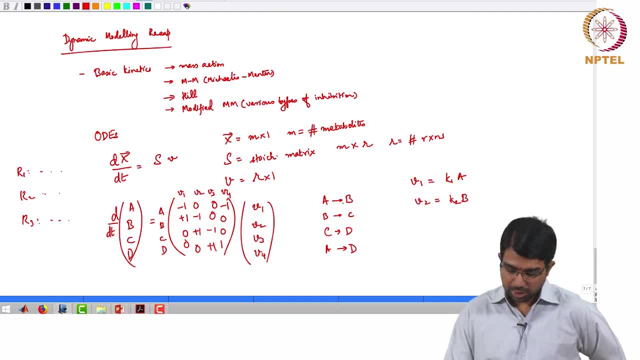 If something is reversible, then you have other things to worry about. But this is literally your entire framework. This is all you need to know for dynamic modelling, right? You have a system of reactions. You write it out in this form. You then for each individual velocity. 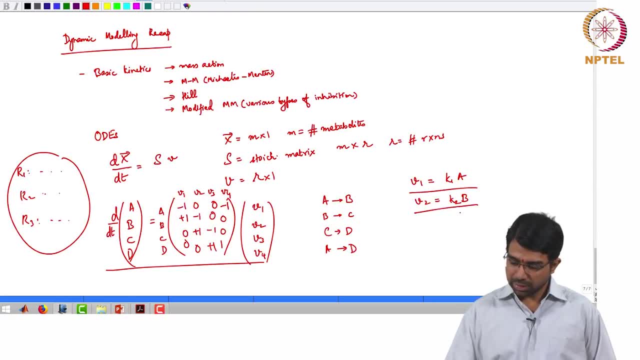 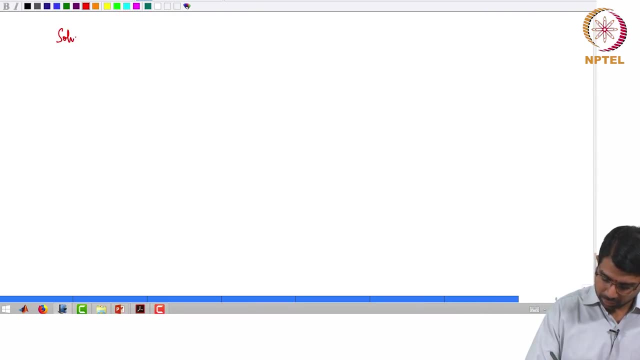 FIRST NEW STATEMENT. See, you can compute it in this fashion and you stick all these back into these equations, your differential equations, and then solve the ODE's. How do you solve them? You have Euler methods, you have Runge Kutta methods- best. 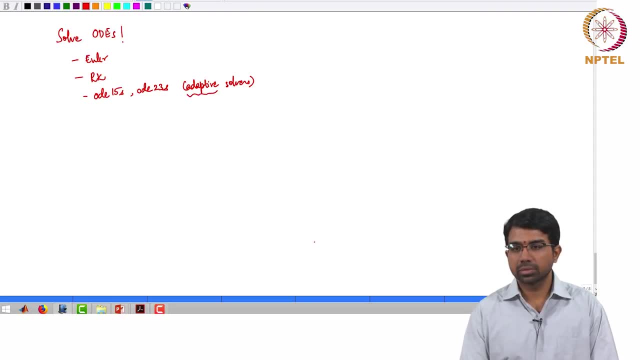 What is adaptive? Varying delta t, Varying delta t, Right? So all your methods basically use some f of x plus delta t, minus f of x by delta t, and so on, Right? Or rather, we would say: f of x, dx by dt equals f of x, equals x of t plus delta t minus x. 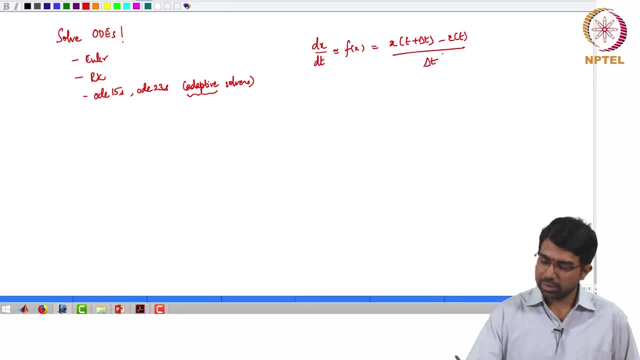 of t by delta t. You use this and the x0 value to predict x at different places. So you essentially have to reconstruct the curve based on the slopes known at different points Right. So for this you use several Solvers. 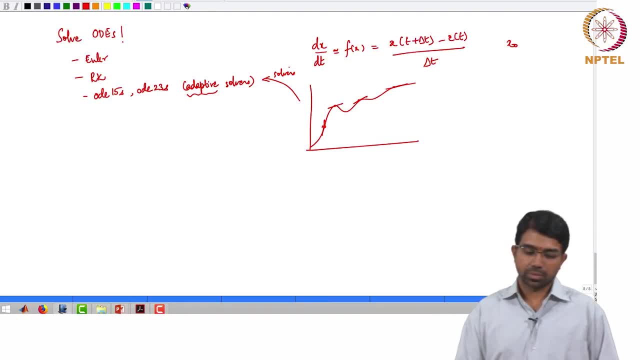 Fair enough. And you also have to worry about stiff equations, which is what these solvers are good at taking care of. So stiff equations typically involve you know several time scales, so you need to have you know the varying delta t's to actually combat them. 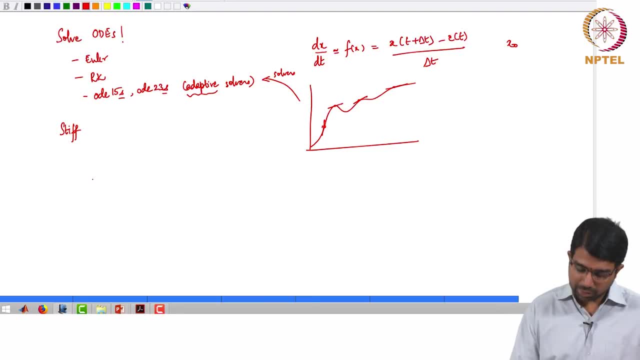 Right. And then we looked at cost function. We basically said we have to worry about several things. First thing is, as one of you mentioned, trends in the data. I might be more interested in trends in the data rather than just the data. and we said: 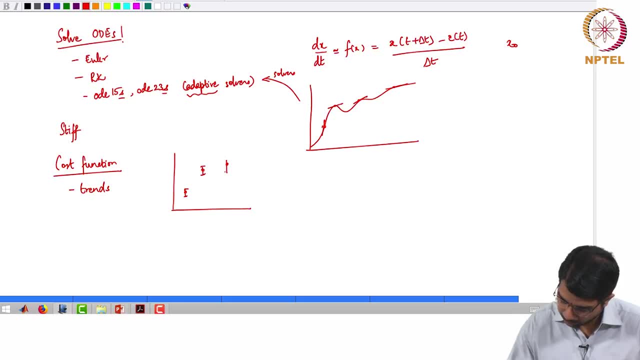 suppose your data points are like this. I will not say that this is the best curve. All these curves, okay, both these curves are equally good. Now, maybe the first one passes through the means, but the second one passes more or less close to the standard deviations, at least. 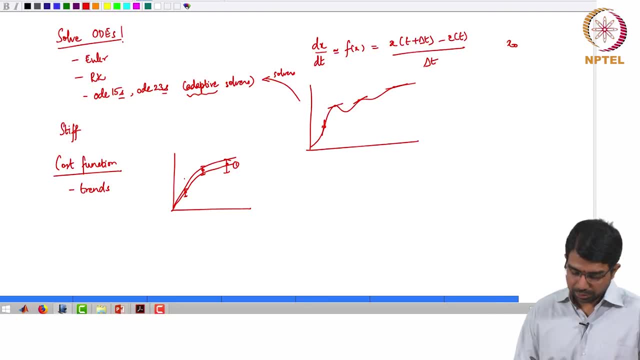 Right. So both of them capture the spread of the data. So we had to account for the varying standard deviations, Varying standard deviation at different points. First thing is scaling right. So we said we will do Xmi minus Xpi theta by Xmi right. 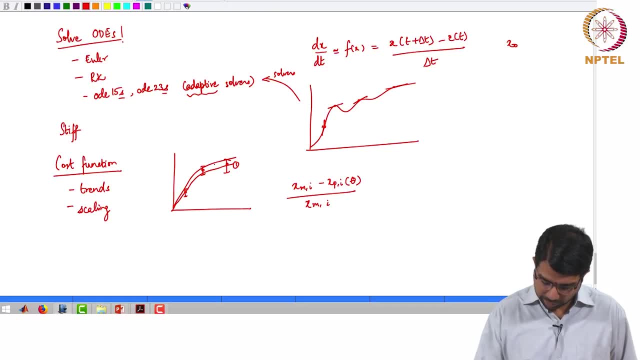 We said, that may not be good enough. so different points may have different error bars, so you want to account for that, and you may be less worried about the steady state than the initial action, So you may want to put something else to account for that as well, and we will square. 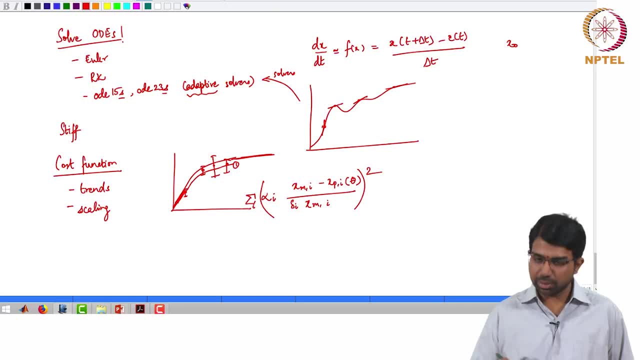 this and sum across all the data points. This is your error. cost function for any given parameter set: theta. How do you find these parameter sets? Okay, Parameter estimation or optimization: We looked at a battery of methods, especially focusing on evolutionary algorithms, right? 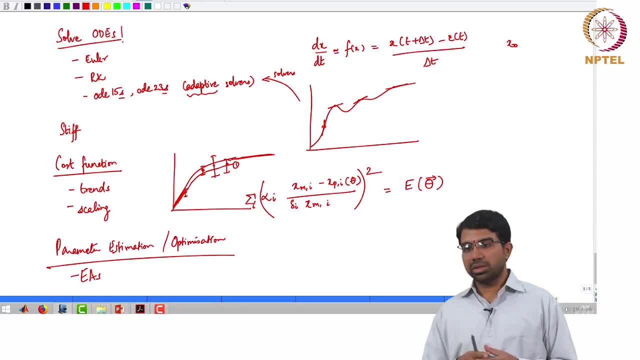 So this in some sense encapsulates dynamic modelling and there are- there is actually another nice NPTEL course on dynamic modelling by Biplab Okay, Which I think you can take a look at because it pays specific attention to, say, modelling signalling networks. what are the? you know, how do you model? positive feedback, negative. 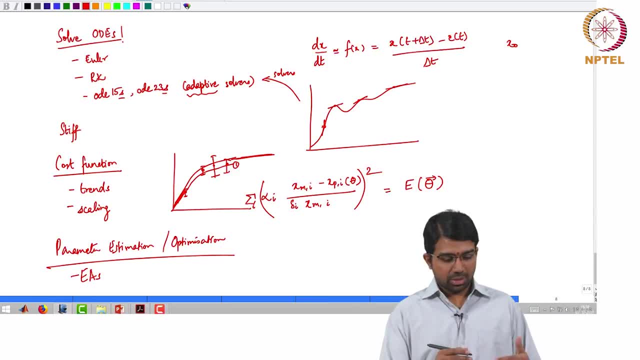 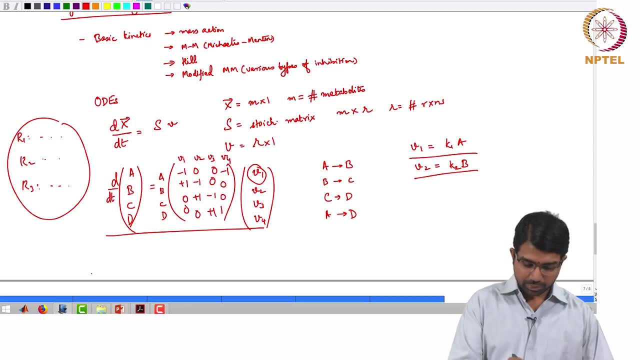 feedback, those kinds of things in greater detail Here in this course. what we have essentially looked at is: there is, you know, a method to model these systems. You essentially set up these kinds of equations, apply the appropriate kind of kinetics for